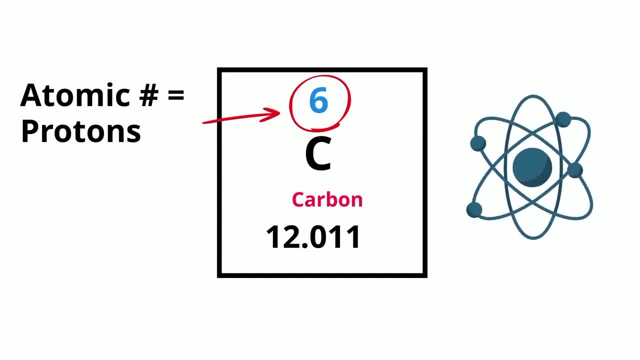 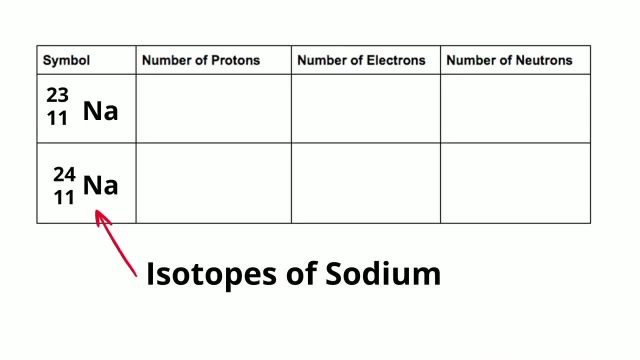 The sum of the number of neutrons and the number of protons in a nucleus is called the atom's mass number. So let's look at sodium 23 and sodium 24.. They both have 11 protons and 11 electrons, which gives them a neutral charge. 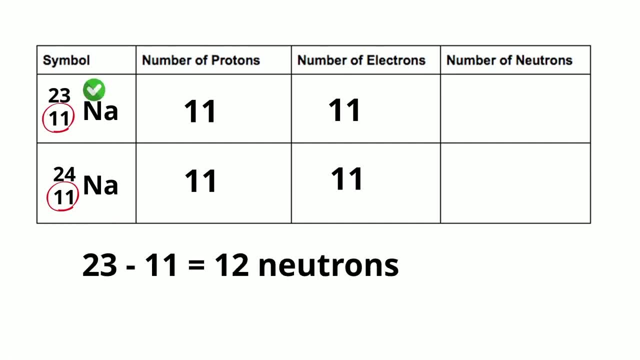 Now for the neutrons. Sodium 23 has a mass number of 24.. Sodium 24 has a mass number of 23 minus 11, which is the number of protons, which equals 12 neutrons. The second sodium- sodium 24, has a mass number of 24.. 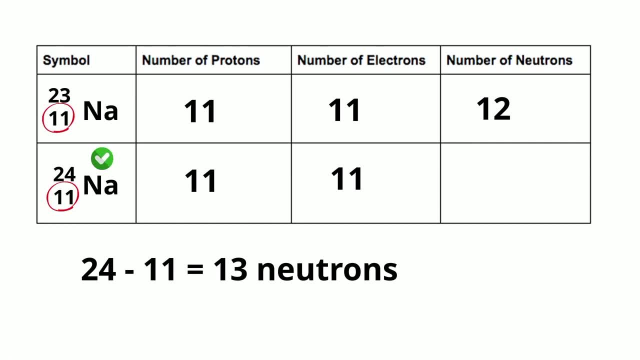 Subtract the atomic number of 11 and it equals 13 neutrons. Let's look at another example. You have carbon 13 and carbon 14.. Both carbons have 6 protons and 6 electrons. Now for the number of neutrons. 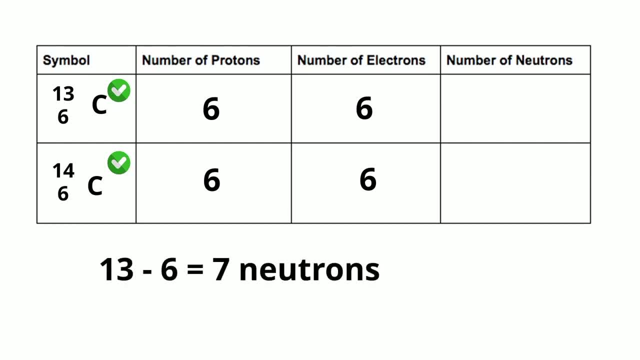 Carbon 13 has a mass number of 13.. 13 minus 6 equals 7 neutrons. 6 is the atomic number And for carbon 14, you take a mass number of 14 minus the atomic number of 6 and you get. 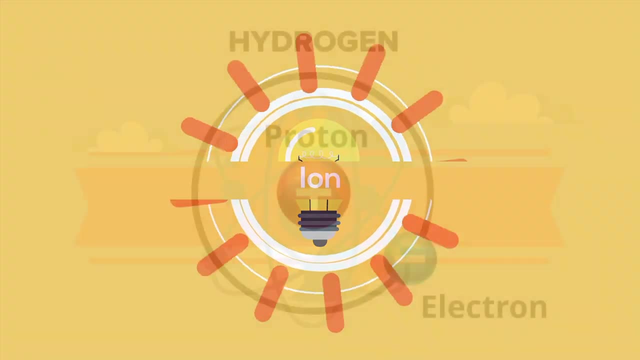 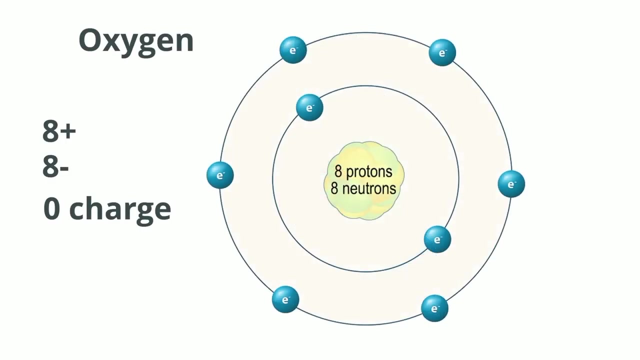 8 neutrons. Let's take a look at what an ion is. An atom will have a certain number of protons and an equal number of electrons. This results in the same number of positive and negative charges, which we can call neutral or a zero net charge. 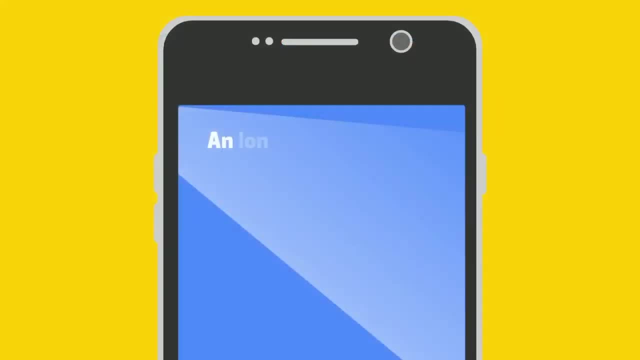 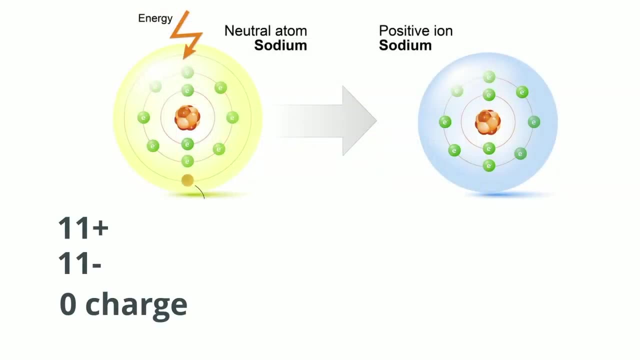 You can produce a charged atom by taking a neutral atom and adding or removing one or more of the electrons, Which is called an ion. For example, a sodium atom has 11 protons in its nucleus and 11 electrons. If one of the electrons is lost, there will now be 12 positive charges, but now only 10. 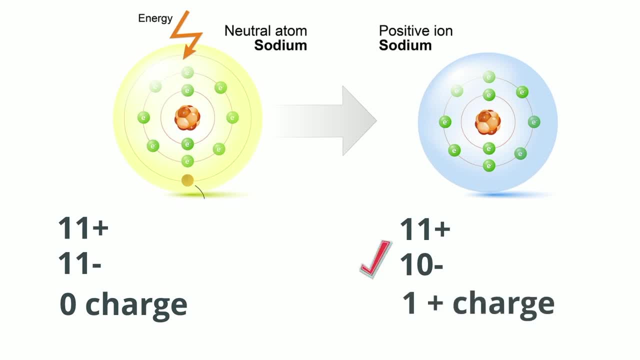 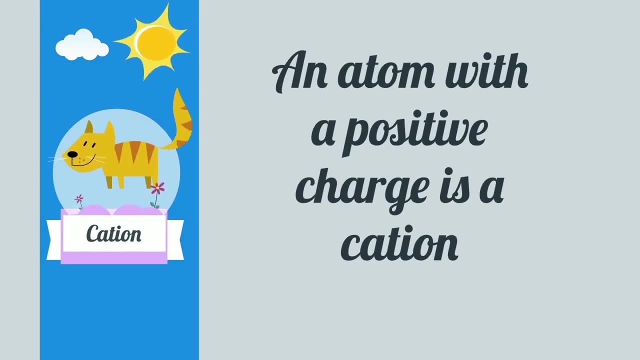 negative charges, so it will have a plus one charge. The sodium ion can be written as follows: A positive ion is called a cation and are produced, as I said, when one or more electrons are lost from a neutral atom. Helpful hint. 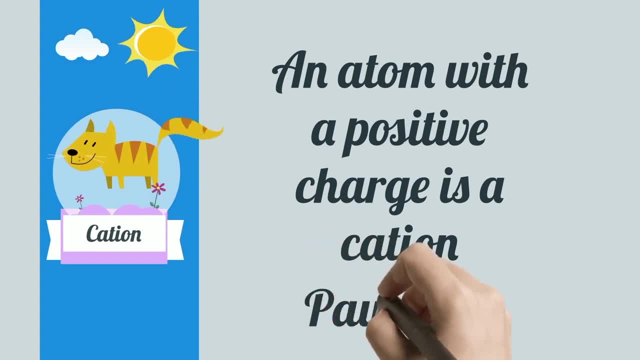 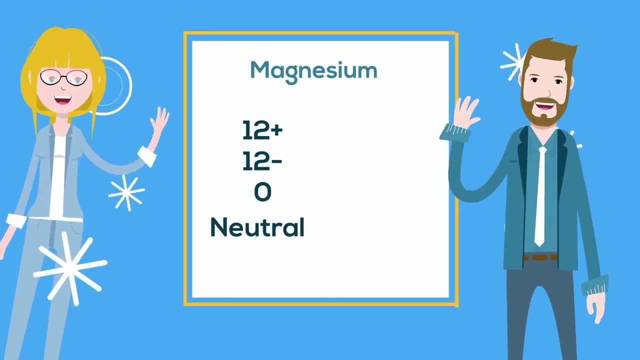 Think of a cation as a cat: It has paws. pause, you know, for positive. Another example: magnesium will typically lose two electrons to form a two plus cation. Neutral magnesium has 12 positively charged protons and 12 negatively.